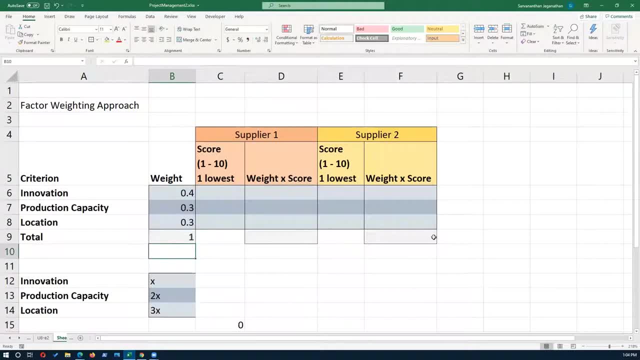 so let's do a quick check. so that is adding up to one, and once you have the weight, now we're going to score each supplier based on these criteria. so you can score. you can use different scale here. I'm using one to ten, you can use one to five, you use one to hundred. 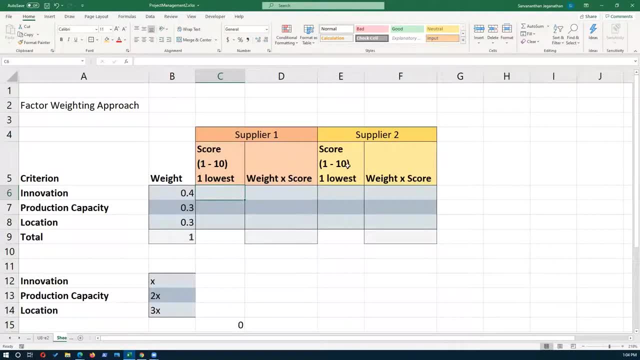 doesn't matter, but it's. what's important is that he uses same scale for different items or different suppliers that you're trying to compare. so here, uh, let's say i give innovation. let's say six out of ten. uh, production capacity, let's say we give a five. and then location is: 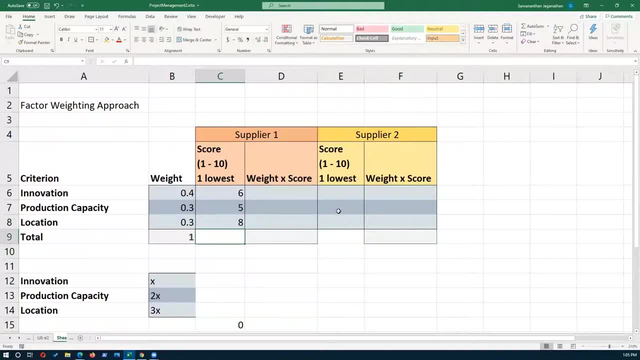 eight, and for this one you go and score. uh, give a score for each one of these criteria. let's say for innovation, say five, production capacity four, and then location, let's say six. so based on this goal, we can calculate the total score. so before doing that, you need to multiply each. we have to 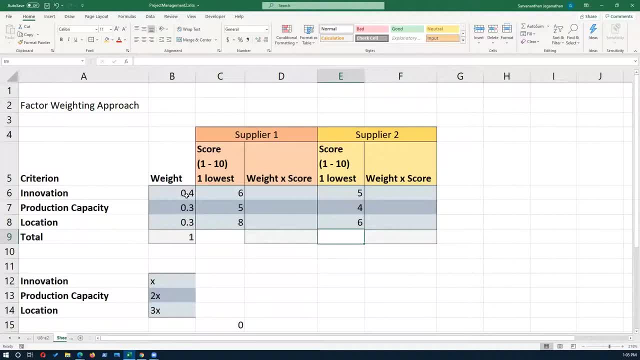 different priority for each one of these criteria. so you need to multiply by the weightage, that the priority is given by the weightage. so let's do that. times the score, that gives us the total of 6.3 for supply one. so similarly you find the total score for: 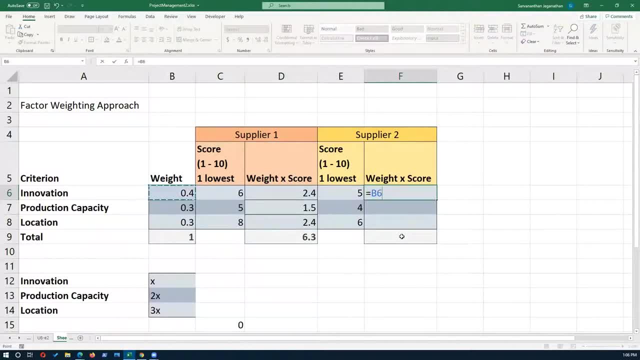 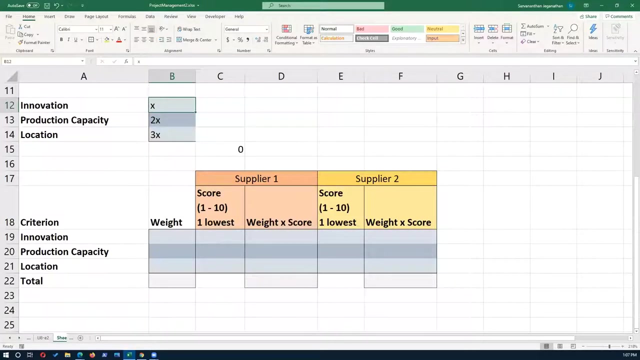 supplier two: that is going to be weight times, the score that you're given and that gives us a total score of five. so in this case the supplier one has the highest score, 6.3. so we would choose supplier one. sometimes in your exercises you might find: 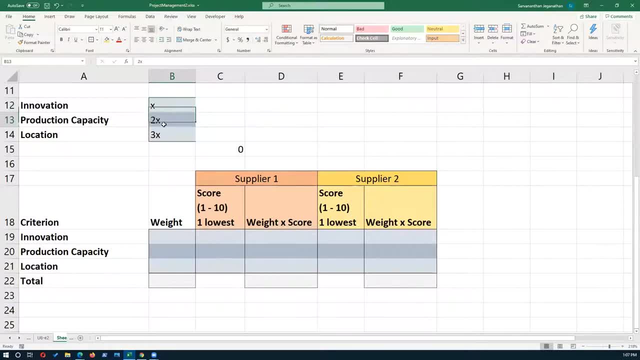 that production capacity is twice as important as innovation, or location is twice as important as innovation. in that case we can use a variable here. so we have x as innovation, and then production capacity is 2x, and then location, its weightage, is 3x, and so on. 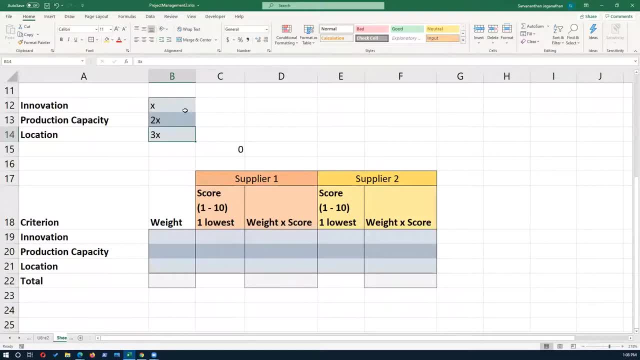 now for our final goal. Now for us to use it in a settings table like this. you need to convert this, find out what x is, So you can create a simple formula like this. So x plus 2x plus 3x here should be equal to 1.. 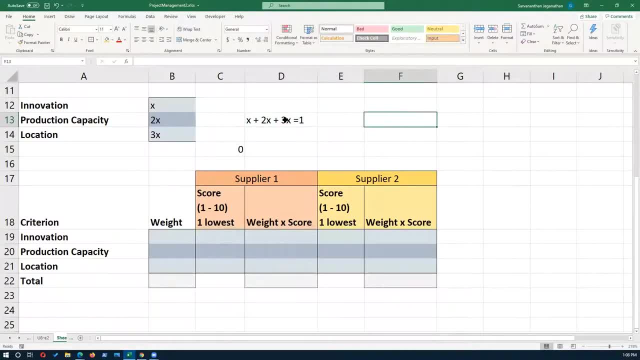 So in that case, if you just evaluate that, that will give you 6x is equal to 1.. And that means x is equal to 1 over 6.. Now you can put that weightage here. So let's find the weightage for that. 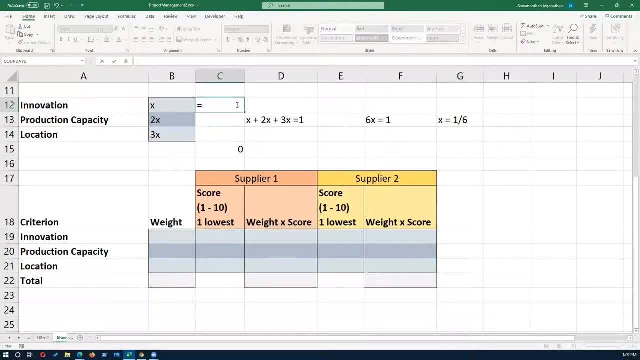 So if x is equal to 1 over 6, we can just convert it into decimals, So it's 1 divided by 6.. That's That's around 0.166.. And then for this one it's equal to 2x. 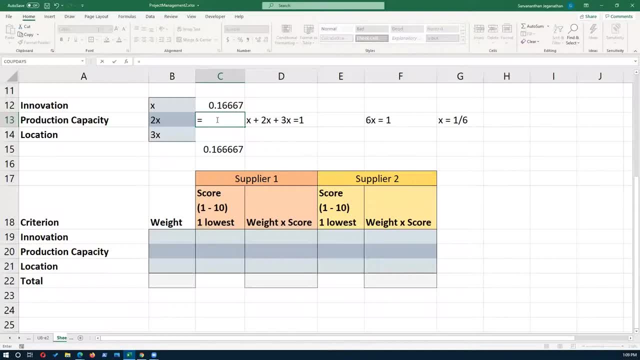 So x is equal to 1 over 6.. So we can do the math here. So it's 2 into 1 divided by 6.. So that's around 0.33.. And same here, equal 3 into 1 over 6.. 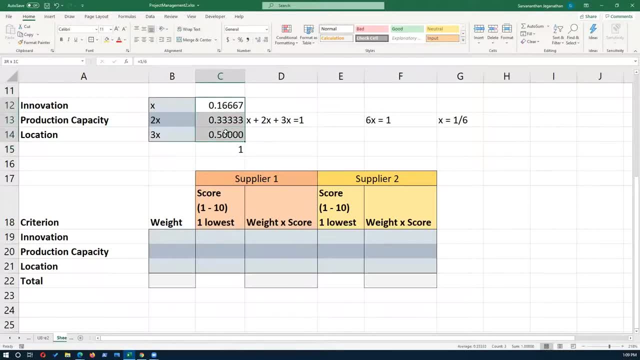 So that's, that's adds up to 1, right? So when you add them all together, that should give you 1.. We can use this weight to do the calculation now. So once you have this, you can get the score. 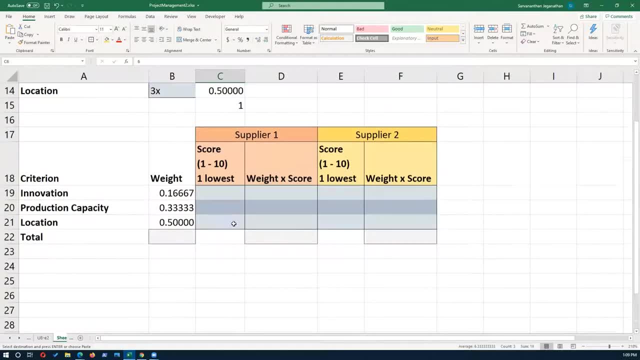 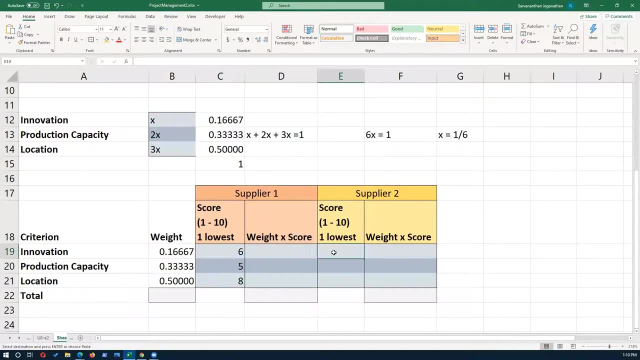 So the score, we have it. We can use the same score. Let's say you can put your own score there And let's say you get the same score, but the weight is different, because This is how we found the priority or weight of each one of these criteria.